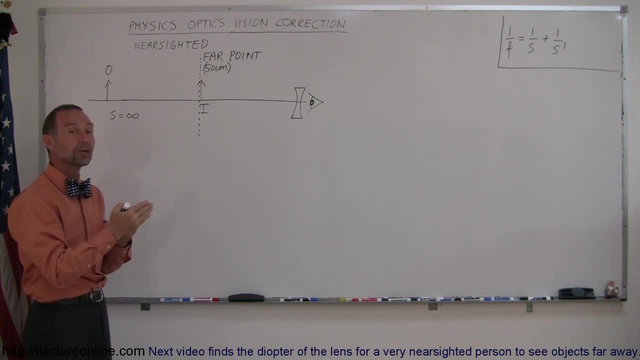 or that person has a far point. A far point is the farthest point that the person can see things clearly, and in this case it's 50 centimeters, which is just a little bit shy of two feet. So as the farthest the person can see clearly is this far, anything beyond that? 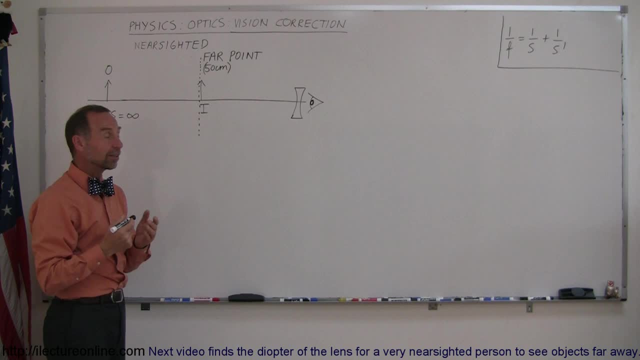 it becomes unfocused. So the objective then is to put some read – not reading glass, but correct the vision glasses on with a diverging lens. that will cause an object that is very far away, and so we say it's at infinity. of course it's not really at infinity, but relatively far away. so that is. 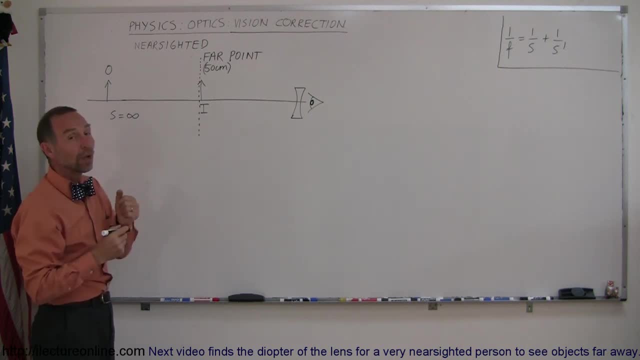 as well as it is using the lens equation, it acts as if it's as infinity and we want to bring to a conclusion that the center of the object is a far point. so let's say we're saying, bring the image of that over here just inside the far point, so the person can see that image. 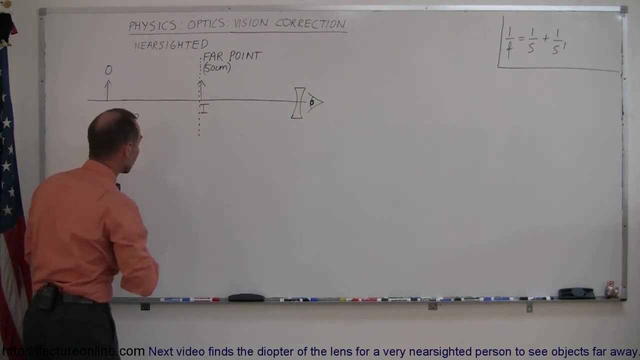 clearly. How do we do that? Well, let's use the lens equation We have: 1 over f is equal to 1 over s plus 1 over s prime. Of course, s is the object distance, s prime is the image distance and f is 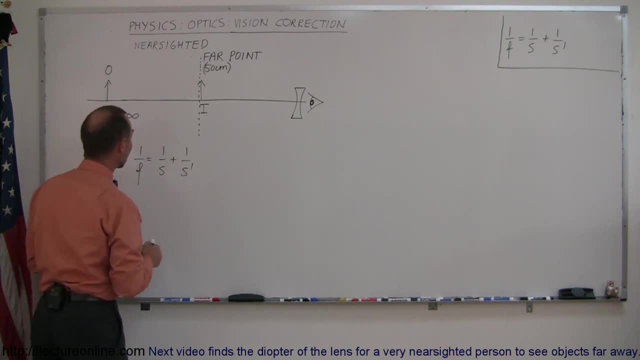 the focal length. So we're trying to find the focal length of that lens. Now let's plug in the numbers that we have For s. we're going to plug in infinity. Now, we don't have to plug infinity. 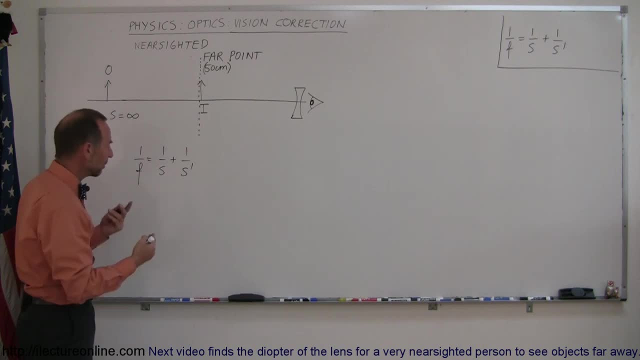 We can put in like 100 feet or 200 feet or 1,000 feet, but infinity works a little bit better. So 1 over f is equal to 1 over infinity plus 1 over s prime. Now s prime is the image distance. 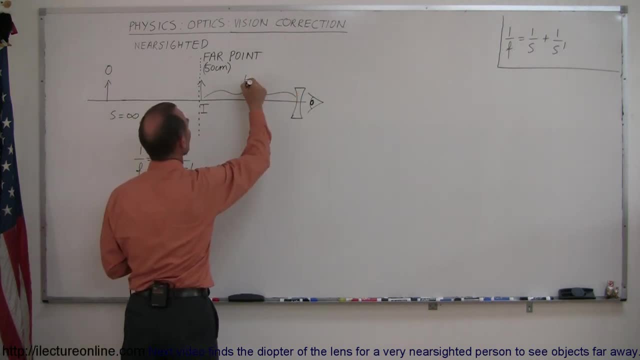 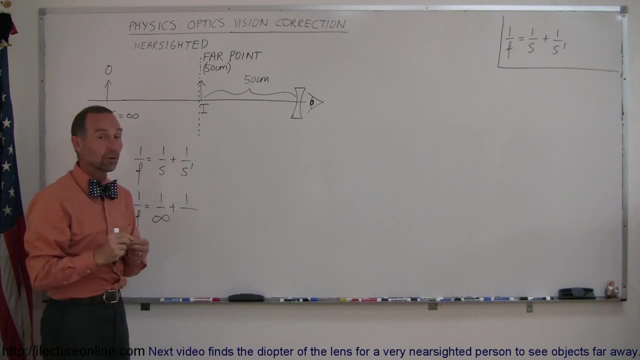 and of course that has to be 50 centimeters. But notice also that the image is in front of the lens, which makes that a virtual image, which means that the image distance is a negative distance, So s prime is a negative 50.. 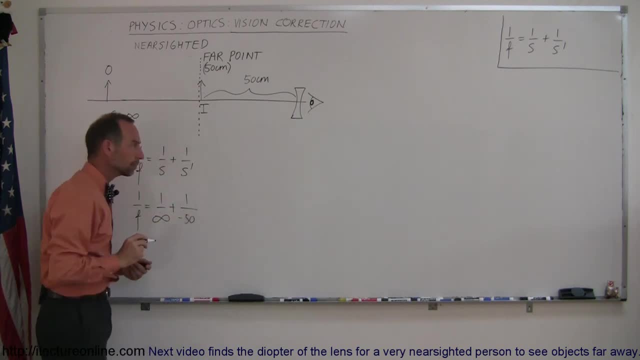 So we plug in a minus 50 centimeters. It's a virtual image. That means people who have corrective vision. if they're nearsighted and they put on a diverging lens, they're actually looking at the world through looking at them as virtual images. All right, Now calculating f 1 over infinity is. 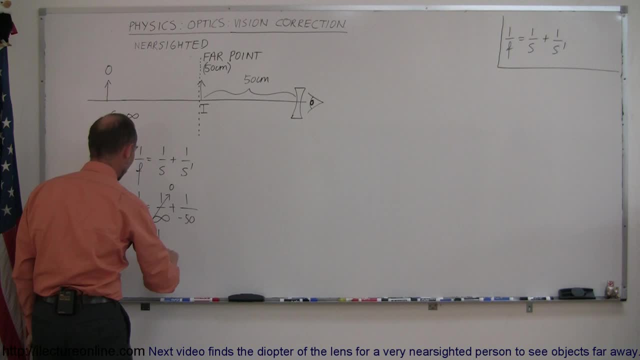 of course 0, because anything divided by infinity is 0. So that means that 1 over f then becomes 1 over minus 50.. And of course then we get 1 over infinity. So that means that 1 over f then becomes.